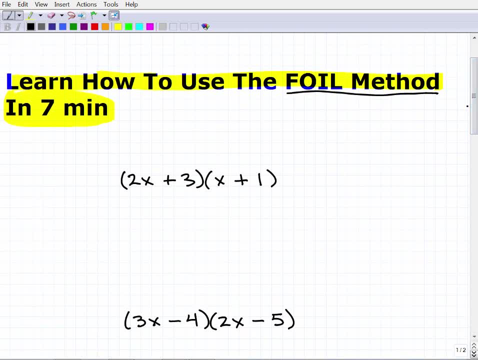 then you should be in good shape with the FOIL method. But Before we get going we need to know what is the FOIL method and why do we need to know it. So this is really a big part of algebra, and in algebra we have these things called polynomials. 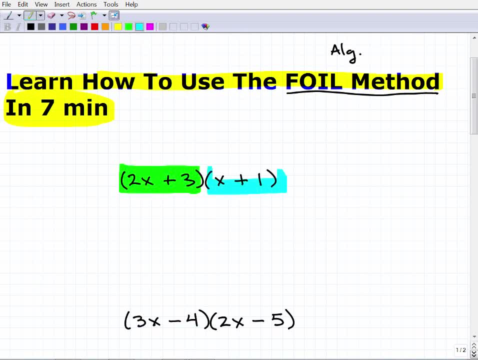 So this is a polynomial and this is a polynomial. Now, these two polynomials. here we happen to be multiplying. but we could take these polynomials, we can add them, we can subtract them and we can multiply them. Then there is something we can do later on, called dividing polynomials. 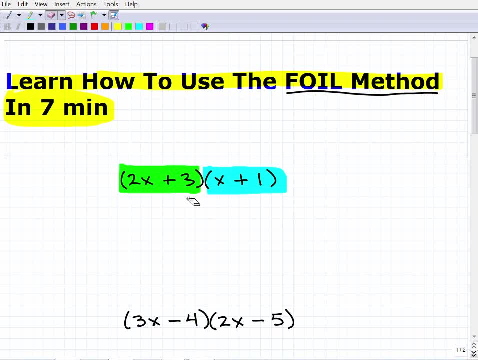 But That's a little bit different. but essentially what we can do is we could. when we have two different polynomials, we can do various operations with them. in this situation, here We're going to be multiplying polynomials, So FOIL has to do with multiplication of polynomials, but not any kind of polynomial. 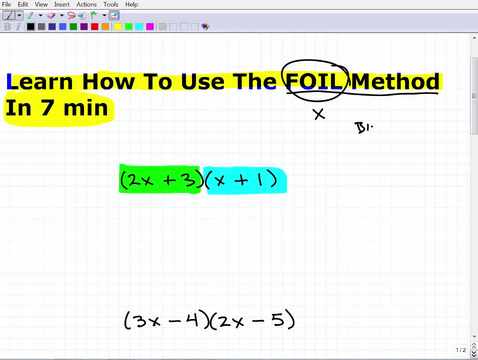 Okay, Specifically what we call binomials- hopefully I spelled that right- And a binomial is a polynomial that has two terms. So we have Something here plus something here, or something here plus something here. you could have something subtracted from something. 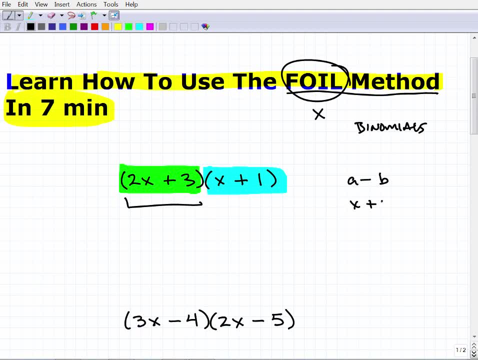 So, for example, you could have A minus B, X plus Y, 3G plus Z. All of these guys here- we could put parentheses around them- are binomials. So we take one binomial, we multiply by another binomial. 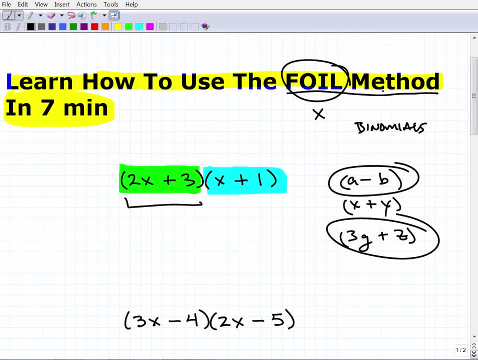 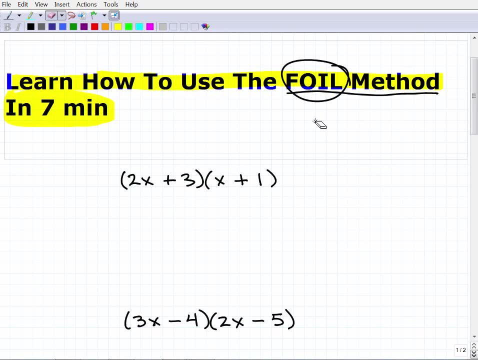 The FOIL method is a specific procedure we follow to multiply two binomials. Now, when you're studying algebra, you need to understand how to multiply polynomials in general. So you could have things like this: two X times three, X squared minus X plus one. 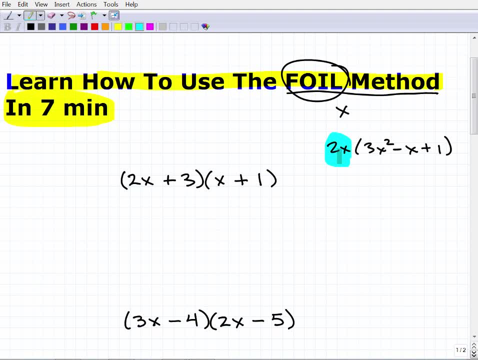 Now this scenario. this is what we call a monomial because it only has one term and we're multiplying it by a trinomial. So in this scenario- scenario- we would not use the FOIL method. Okay, Remember, the FOIL method only applies to a binomial times a binomial. 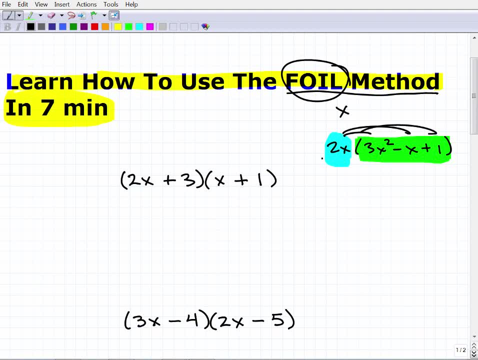 So here you would use the distributive property And then if I had a binomial, times a trinomial. there's other methods that you need to learn, But the FOIL method is a very popular method And, with that being said, now that we know what it is, let's define this little acronym: FOIL. 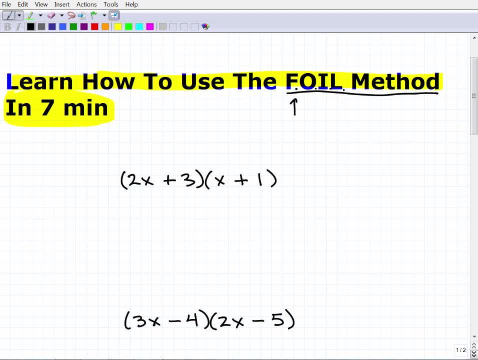 This really should be FOIL. So the F is first, the O is outer, the I is inner And the L is last. Okay, So I'm going to demonstrate this problem because, again, my objective is to teach you this stuff in a pretty short period of time, hopefully around seven minutes. 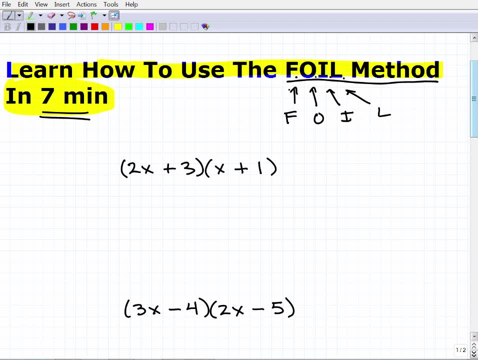 But you know, the video is no good if you don't learn anything from this, right? So the FOIL method, this is the procedure. We're going to do the first, then we're going to do the outers, and then we're going to do the inners, and then we're going to do the last. 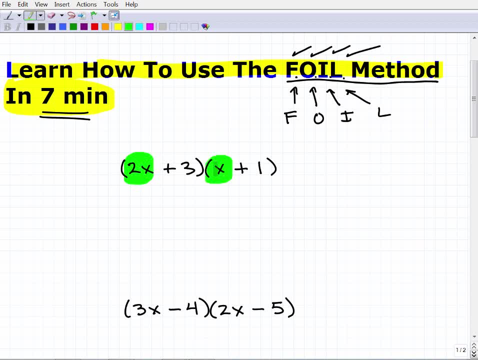 So what is the first? The first is these two guys, Okay. So if you look at each binomial, the first term in each of these binomials are these: Okay. So this is the first, So we're going to multiply the first. 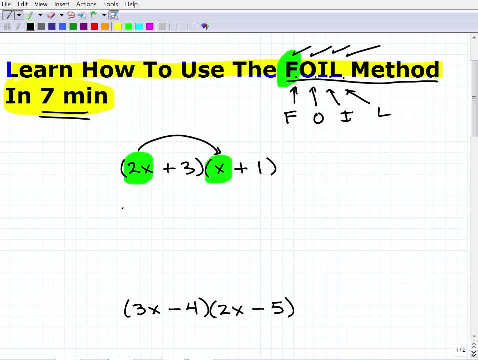 So it's just this: times this, 2x times x, is 2x squared. Now, hopefully, again. if you didn't understand this, then you're going to do some, you know, additional review, But if you're with me, so far, excellent. 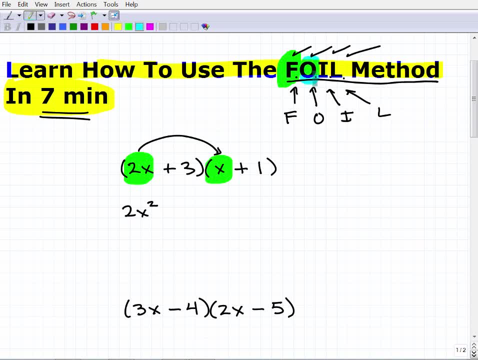 Now we're going to do the outer. Okay, The outer. So we did the first. Let me go back and just kind of keep this here. So we did the first. Now we're on to the outer. So the outers are these guys: 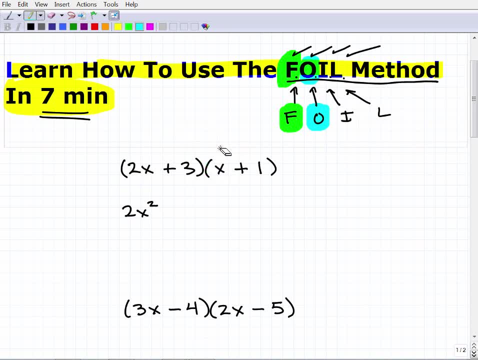 Okay, The outers happens to be: let's erase these. Okay, These guys here. These are the outers. So 2x times 1.. 2x times 1 is simply just 2x, Okay. So if you're with me, you're like: okay, get this. 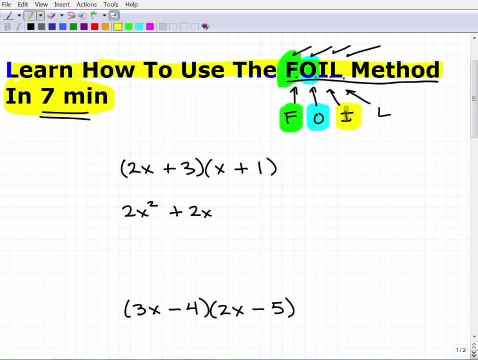 So now we're just moving on to the next one, And the next one is the inners. So what are the inners? These two guys here are the inners, Right. So this is the inners. These are the outers. 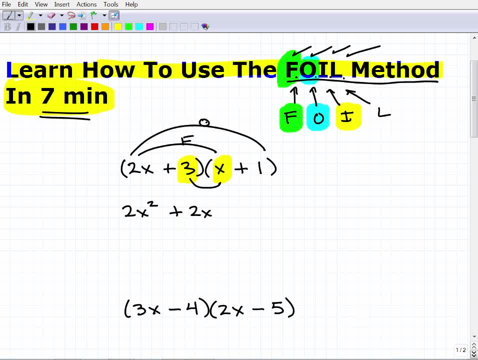 These are the first. Okay, So we did the first outer and now this is the inner. So 3 times x is just simply 3x. And now, notice, I just put an addition sign because we're going to every time we do a little, first, outer, inner, we just take that term. 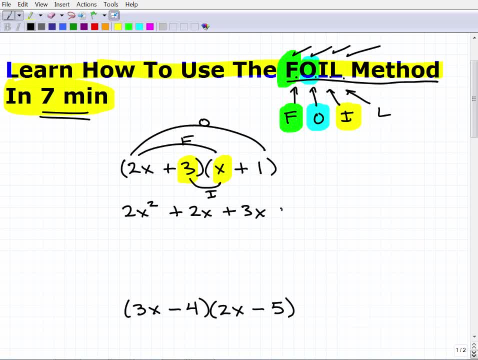 and then we're going to add it to the next thing on a checklist. So the next thing on a checklist is the last. Okay, So if you look here, if you're kind of confused, we say we multiply this times, this, this times, this, this times, this. 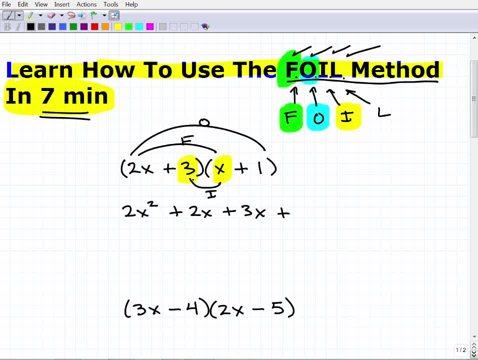 Now the last would be the last of each Okay. Binomial, So that's 3 times 1.. So this is the last Okay, And 3 times 1 is 3. Okay, So now all we have to do is combine like terms. 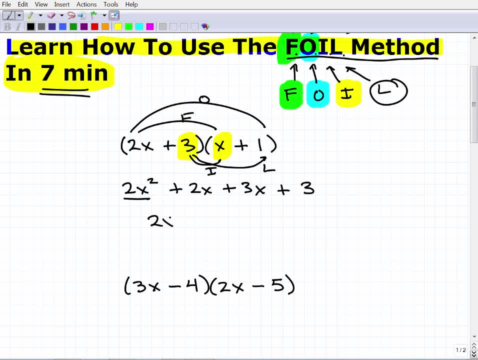 So I have 2x- 2x squared, excuse me- And I have 2x plus 3x. which is what? 5x plus 5x, and then I just have this little 3 remaining, plus 3.. 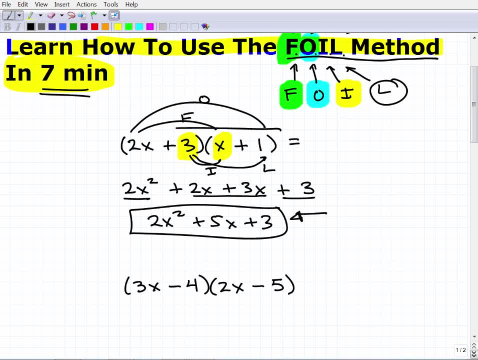 So this is the product of multiplying these two guys together. Okay, So we had a binomial times a binomial. Our brain said, oh, I need to use the FOIL method. First, outer, inner, last. Just do this little procedure, add everything up at the end and you're done. 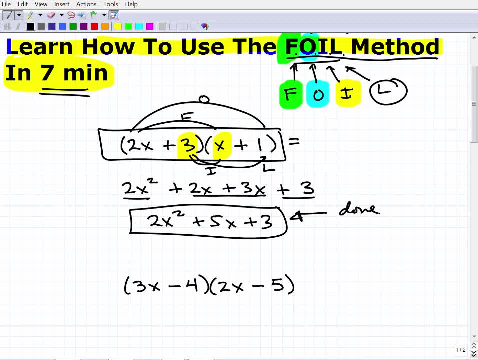 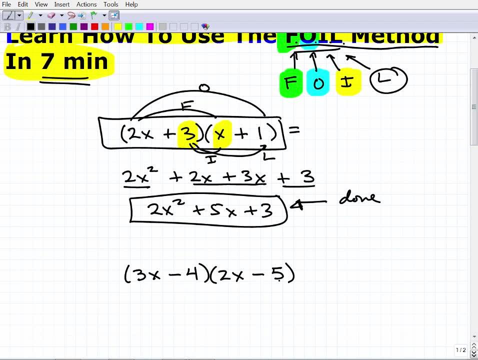 Okay, So if you understand that, why don't you go ahead and see if you can apply your new knowledge on this problem? Now, this problem, I have some subtractions, some differences going on, So you got to be careful here. but if you want to pause the video and give it a whirl, 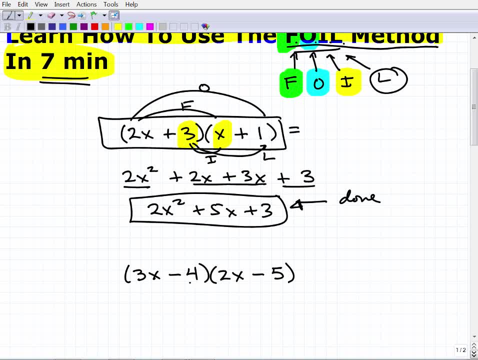 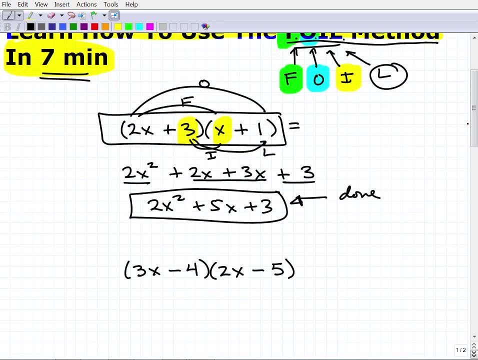 before I do it. Okay, I think that's a good little pop quiz for yourself, Okay. So, with that being said, I'm going to go ahead and do this now. So, if you want to, if you don't want to see the solution, you might want to pause the. 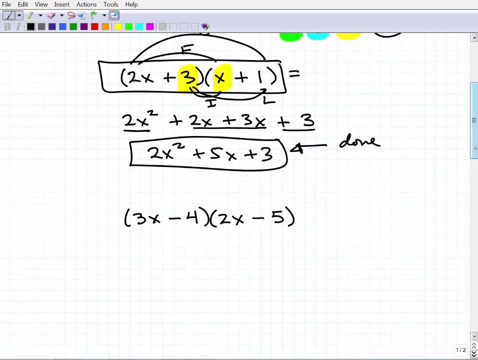 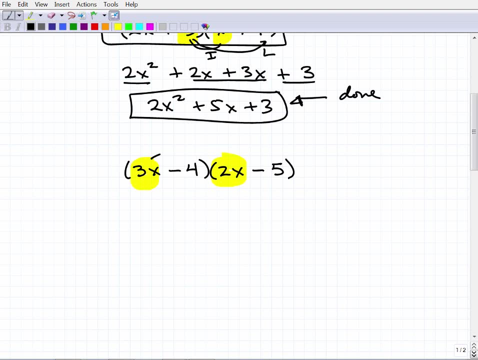 video, but I'm going to go ahead and do it now so we can get this video done in a decent period of time. Okay, So I'm going to do the first. All right, So the first. let's just do it this way. 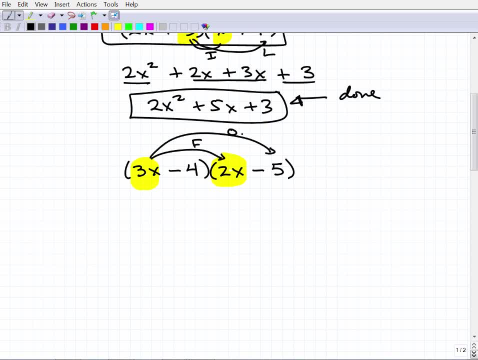 So this is going to be first outer, inner and then the last right. Okay, So now I'm concentrating on the first. That's 3x times 2x, So that's 6x squared. Now the outer is going to be 3x times. now this is where students make an error. 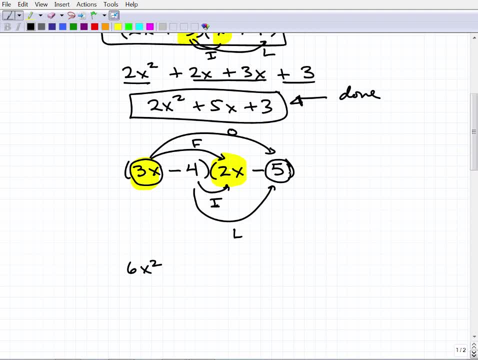 They go: oh, that's just 3x times 5.. So if you said that's just 15x, you were close. Okay, But you're not quite right. Well, you have to include the sign. So this is really a negative 5.. 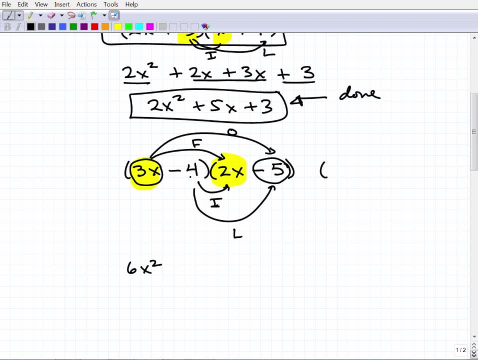 So, if you want to, you could think of this problem. We have 3x minus 4.. You could think of this problem this way: 3x plus a negative 4, if that helps, you see that Okay. So this is really 2x plus a negative 5.. 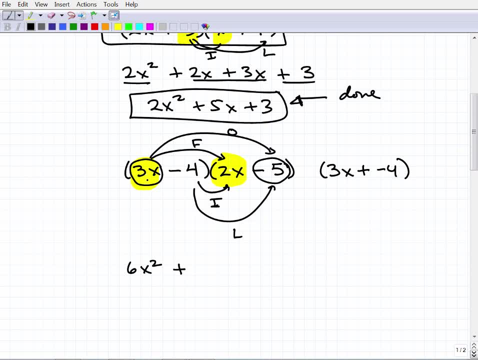 So you have to include this negative sign. So this is going to be plus 3x times a negative 5.. So that's negative 15x, Okay. So, with that being said, let's continue on with the inner. So this is like plus negative 4, right? 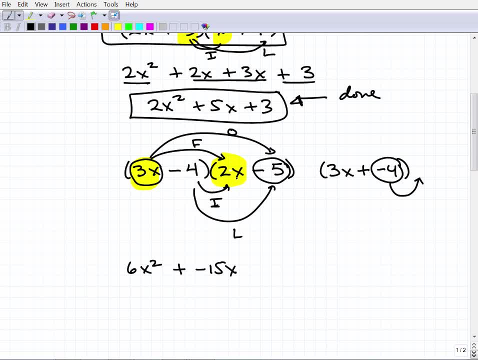 So we have to use this negative 4 to multiply by this 2x, So that's going to be plus negative 8x. all right, Then we'll finish up with the last. That's a negative 4 times the negative 5, which is going to be positive 20.. 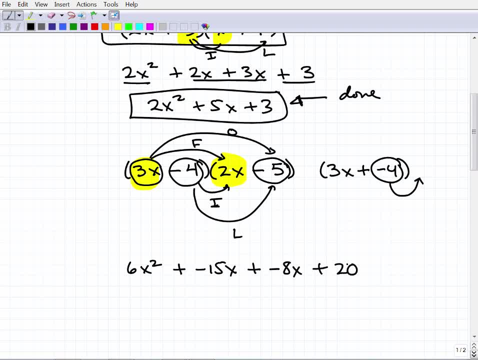 So the negative signs, really, you know plenty of students, you know mess up. They understand the general concept, but when you've got some positive and negative numbers going on, they'll make a lot of errors. And I know that from many, many years of grading thousands and thousands and thousands of papers. 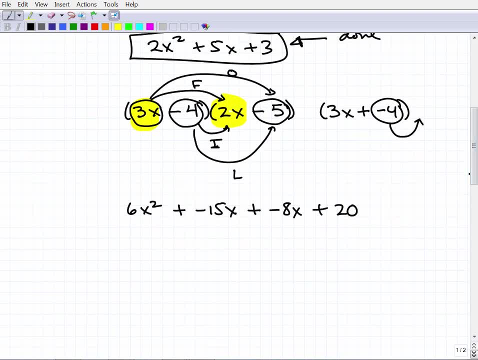 So, with that being said, you get a lot of experiences As a teacher and you know what. I'm sure. way back many, many, many years ago, when I was in school, I was making the same mistakes. but let's go ahead and wrap this up. 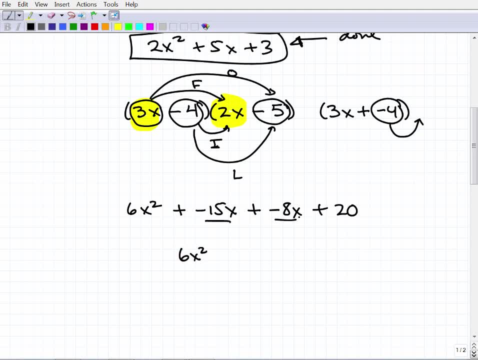 So this would be 6x squared, and then we have 15 and 8- is what? 23,, if I didn't make any mistakes, right? So let's be plus negative, 23x plus 20,, and then I'll be done. 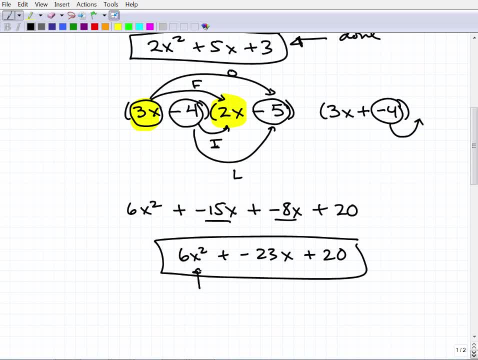 And you always want to write your answers in standard form. highest power of x, that'd be x squared Okay. And then, lastly, your number Okay. So I have no idea how much time I've been on this video, because when I get going, I. 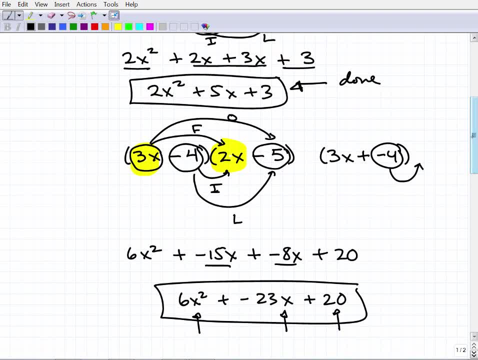 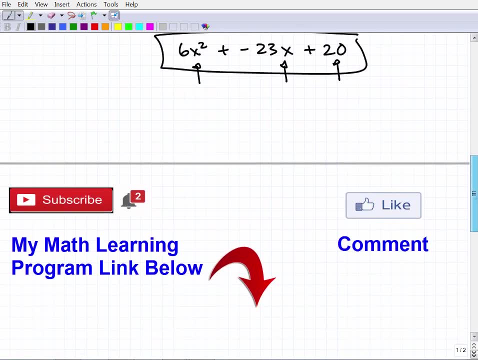 teach to what I think is sufficient. Hopefully, this was a good little kind of power lesson for you and you're like: okay, you know, I got this. now, Of course, what counts is practicing this. all right, You might understand these two problems in a moment, but now you actually have to go.